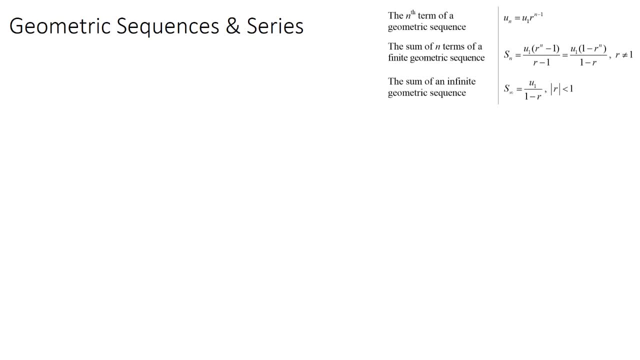 In this video we're going to look at geometric sequences and series. So a geometric sequence is a sequence of numbers that has a common ratio between all of the terms. So the easiest example to do with a geometric sequence would be the sequence 1, 2, 4, 8,, 16,, 32, so on, so on, so on. 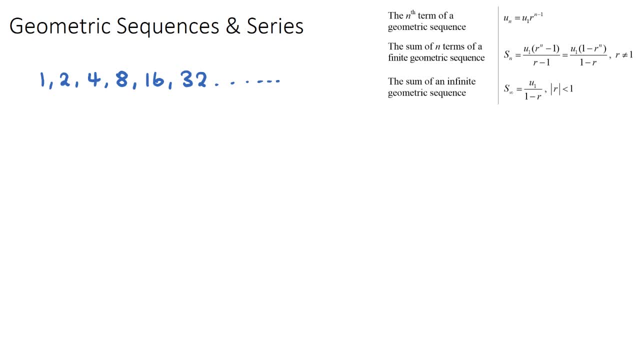 So, unlike an arithmetic sequence where we have a common difference between all of our terms for a geometric sequence, we have a common ratio And we can kind of spot the ratio here, because to get to each new term we're multiplying by 2. And it's going to be consistent. And the fact that it's consistent means that it will be. 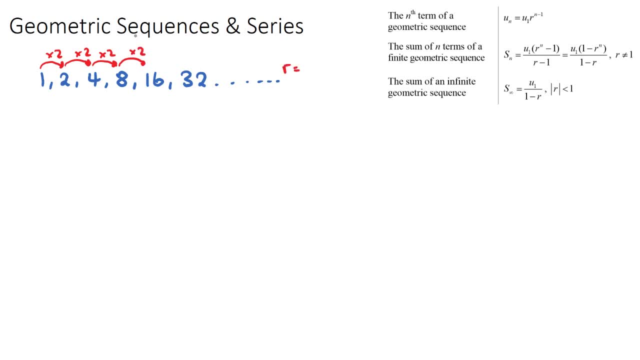 a common ratio and we'll have a geometric sequence. So the ratio here would be positive: 2.. Now there are some formulas, some IB formulas, that they do give us that helps us find any term in a geometric sequence, So we might be able to find the 10th term without having to use our hands. 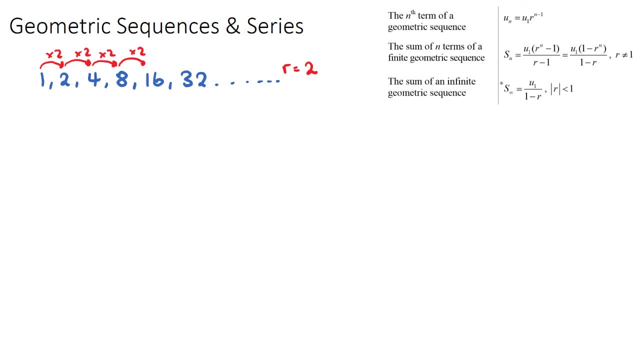